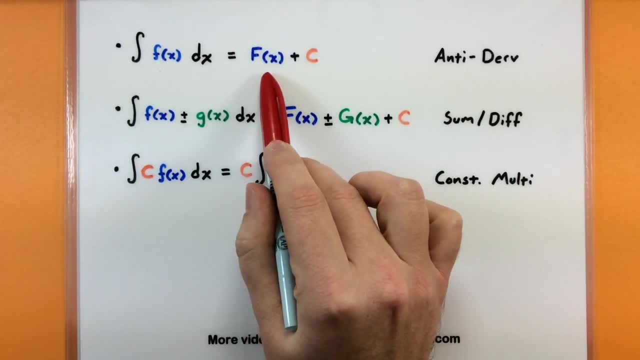 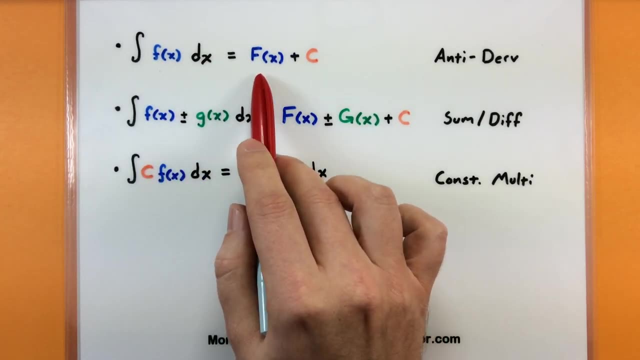 And oftentimes you'll see this. You'll see notation for an antiderivative: simply use a capital letter. So what this is trying to say is that I'm starting with some sort of function, I'm working backwards and its antiderivative is now over here, which I'm calling capital F. 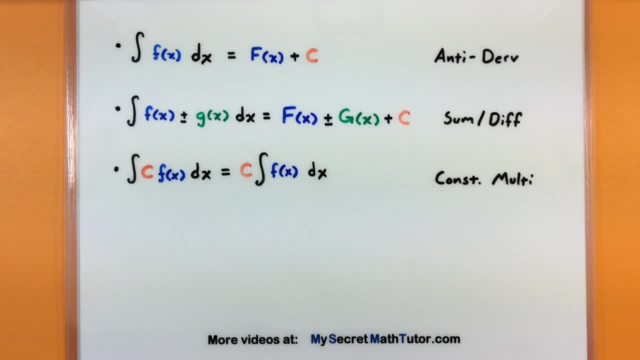 These antiderivatives will also involve a plus C or a constant, And that's because when we're taking the antiderivative it may have some sort of constant component, but usually the derivative wipes that out, so we're not even sure what that is. 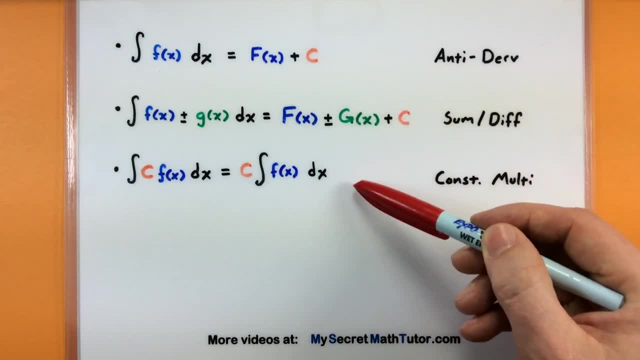 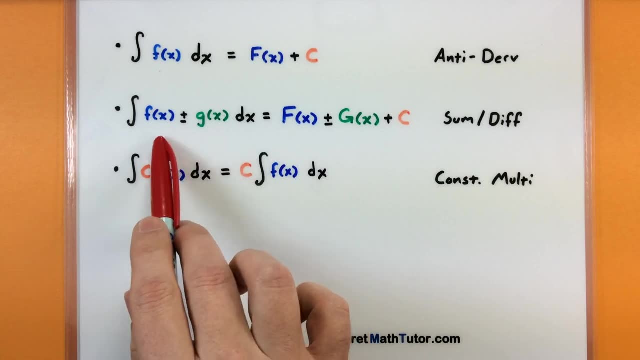 Now, this is probably the biggest thing you have to keep in mind. There are a few other things that are good about antiderivatives or indefinite integrals, and that's they have a sum and difference rule. So if you have two functions that are added or subtracted, then you're simply taking the antiderivative of each of those and adding and subtracting respectively. 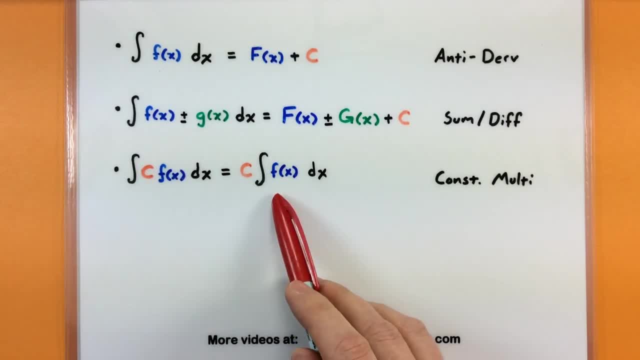 If you have a constant multiplied out front, feel free to pull out that constant. Then you can just worry about taking the antiderivative of the function. that's left on the inside. All right, so there's not a whole lot of rules, and that's kind of a nice thing. so not a whole lot to remember. 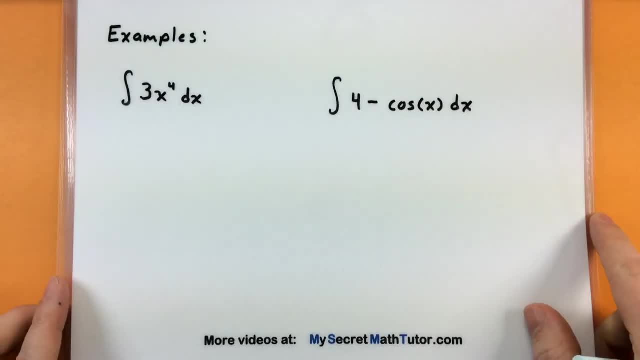 Let's go ahead and jump into some examples and see how they play out. So for the first of these, I'm going to look at the indefinite integral of 3x to the fourth power, And I could also say I'm just simply looking for the antiderivative of 3x to the fourth. 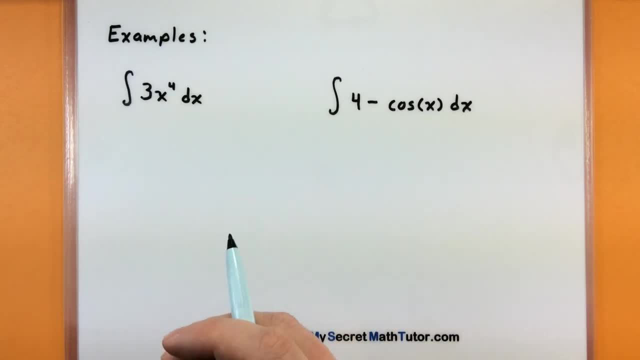 All right. so the biggest thing you want to think of is: you know, if I was to start with a function and take its derivative, then it would turn into this, And to really get good at that process you have to start really knowing your derivatives. 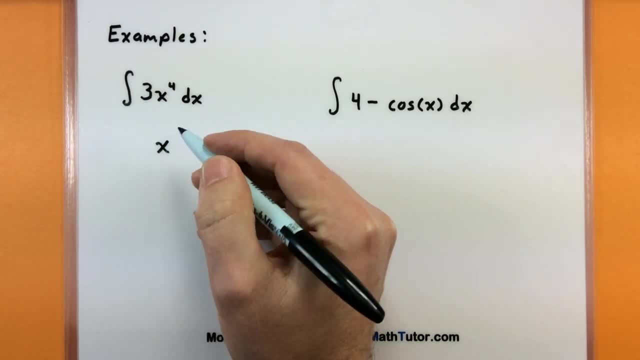 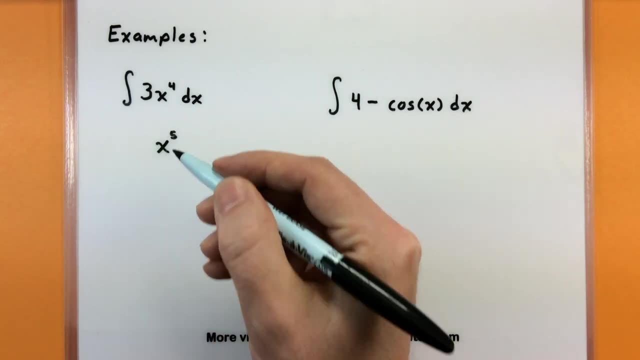 So, for example, I might start playing around saying: Okay, when I take derivatives, I bring down the power and I reduce it by one. So if I was doing that, I think this power must have been five. You know, that'd be the only way that I could reduce it and it would end up as four. 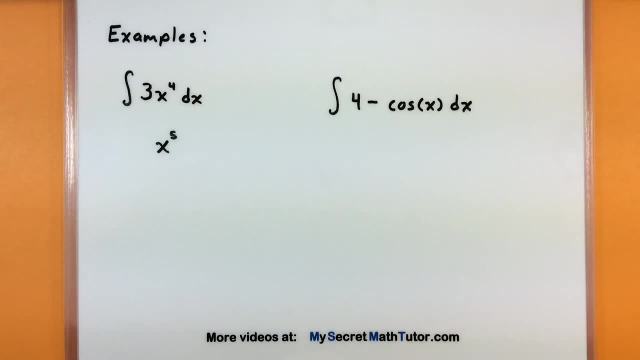 So, in going in the other direction, I would think of like adding one to the power. All right, now the three is a constant, so I'm not going to worry about that. In fact, it's just going to hang out for a bit. 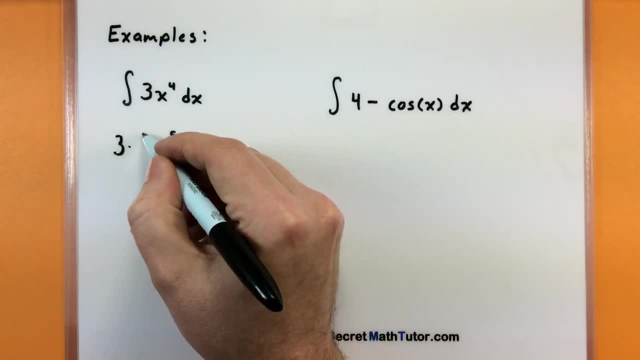 And let's see what should have been out front. You know I'm going to say that that is a one-fifth And then we'll put our constant. So it's a really big process to think backwards like that, but let's go ahead and check. 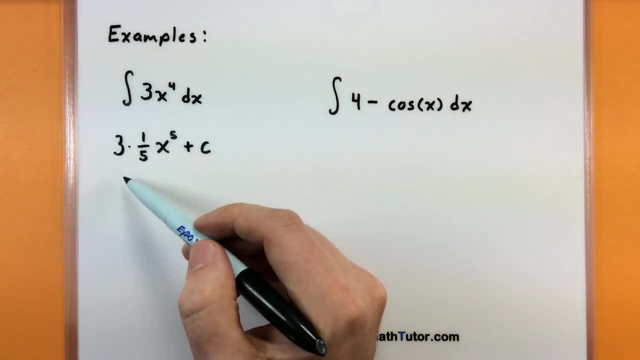 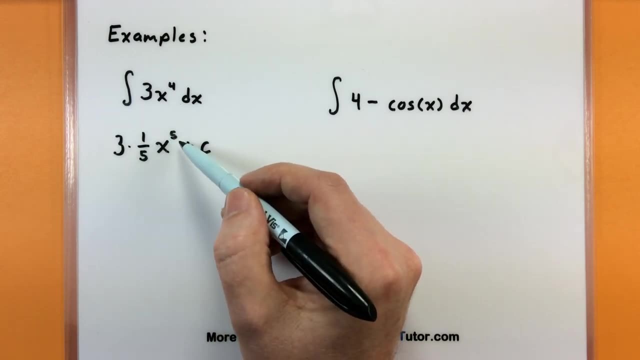 So if I was to take the derivative of this- you know derivatives, they also are not affected by these constants out front, But I would bring down the power. it'd cancel out the five and this would be reduced by one, turning it into four. 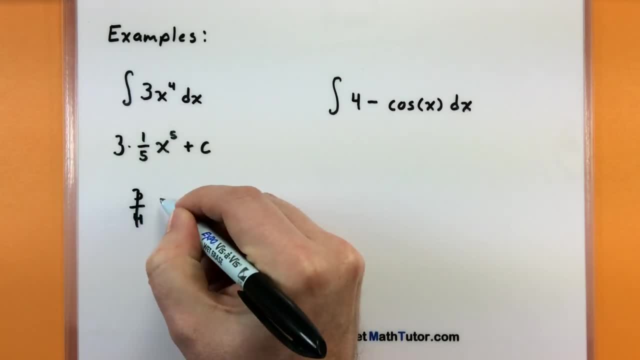 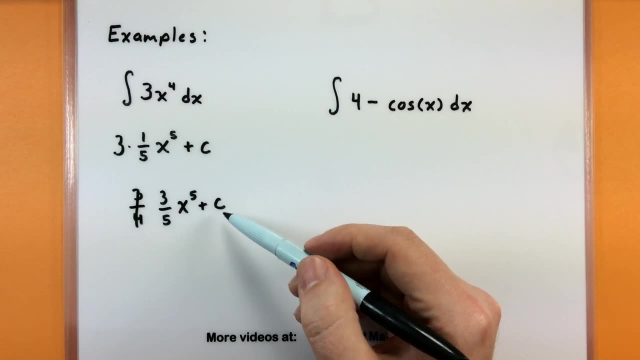 So, sure enough, we see that our antiderivative is three-fifths x to the fifth power, plus some sort of constant, And this is what we would have for the, you know, indefinite integral. All right, let's try this again with another example. 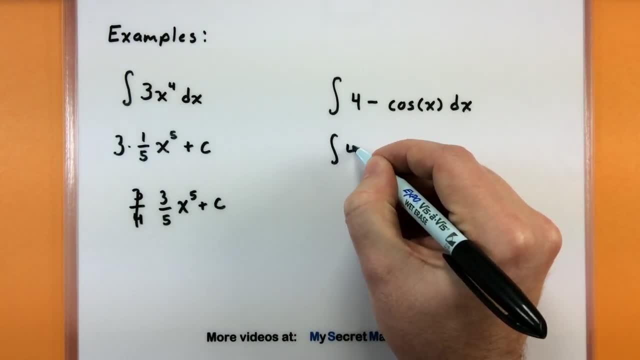 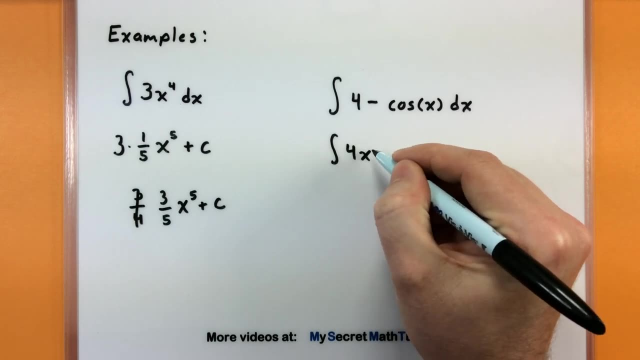 This one. I'm going to try and walk through a little bit more, just so we can see what's going on here. So if you see a constant and it's not being multiplied by anything, you can consider it to be a variable, but with a power of zero. 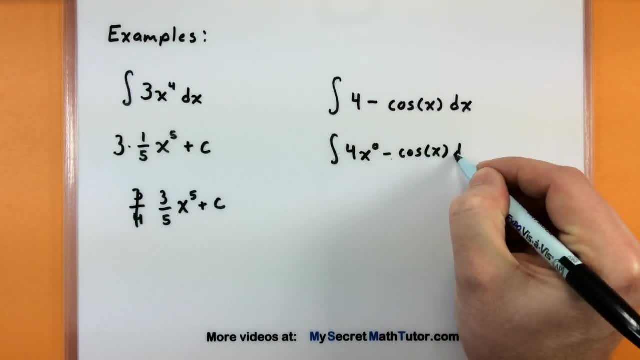 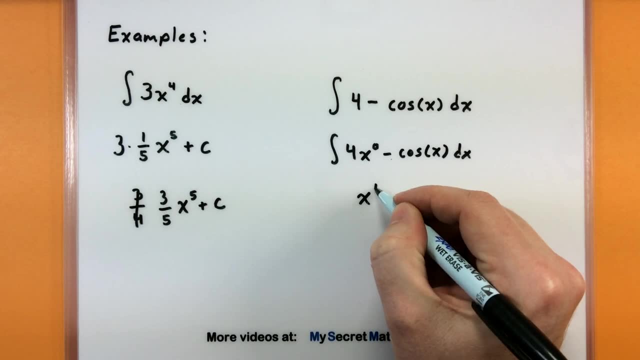 All right, so here's a cosine of x, dx, And again we want to think backwards. So I'm thinking about this power. let's see, I will add one to the power. So zero plus one is one, And then I'm going to end up dividing by this new power. 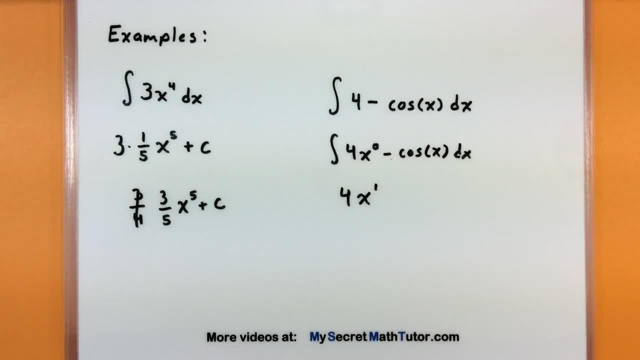 So four divided by one is simply four. So that looks pretty good. Moving on to cosine, what function's derivative would equal cosine? Well, that would have to be sine. Of course we put a plus c on the end. I could clean this up a little bit and just say this is four x minus sine of x. 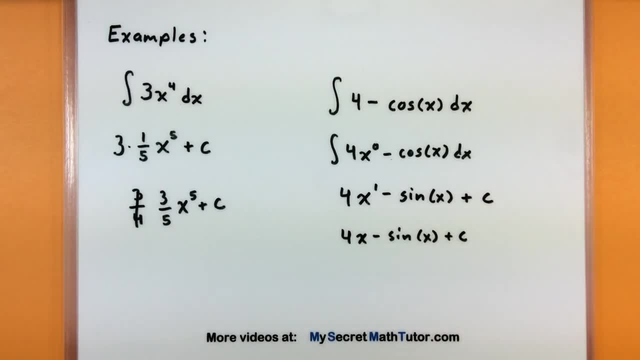 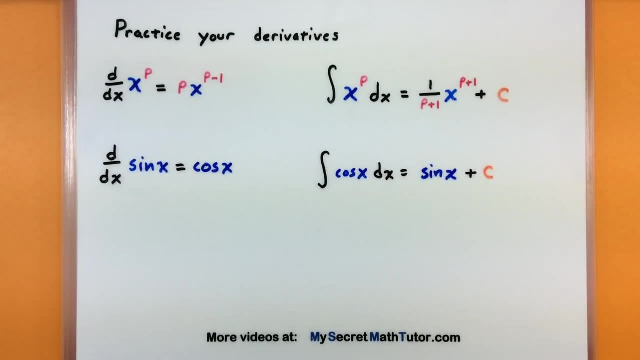 Plus a constant, and that would be my antiderivative. So you'll notice that one thing that can make this a much easier process is knowing your derivatives really, really well. The more derivative rules you have in your back pocket, the better you'll be able to recognize your antiderivatives. 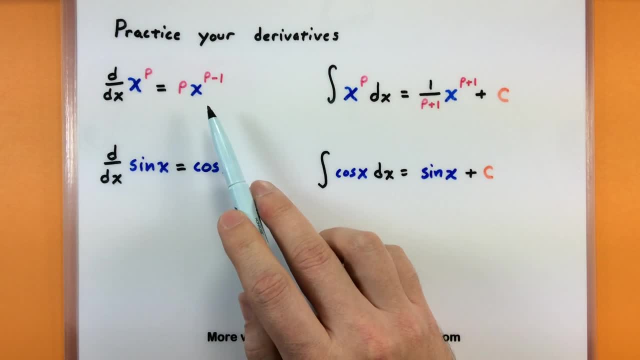 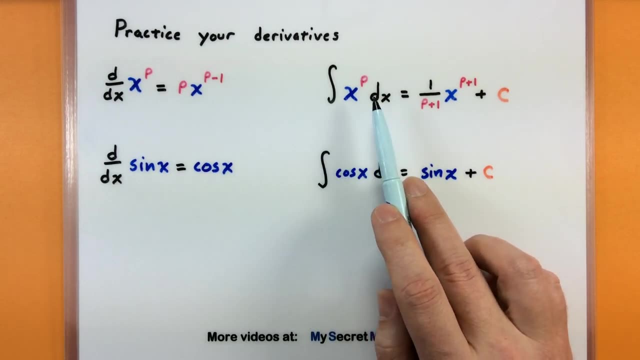 and be able to move in that direction. One of the biggest, though, is probably this power rule for derivatives, And the way you're going to see it show up for antiderivatives is when you have something like x to a power. 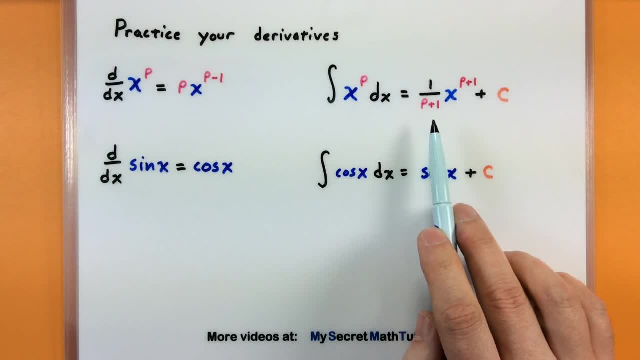 you're going to add one to the power and then divide by that new power. So it's exactly like the usual power rule, but it's doing opposite things. It's adding one to the power, it's dividing by the new power and of course you saw me use that in a couple of the last examples. 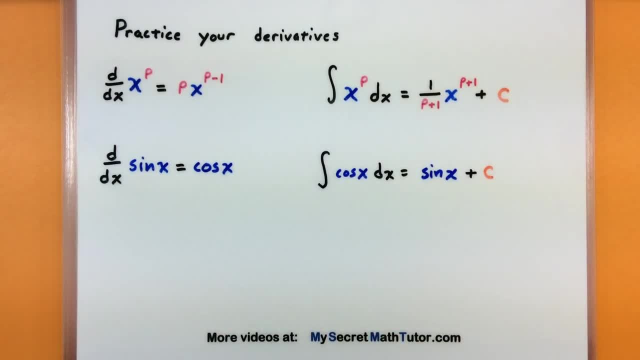 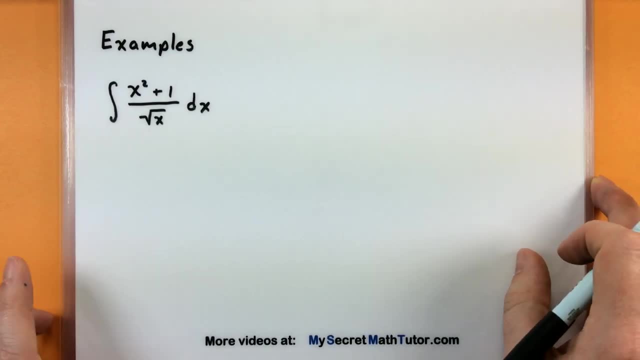 The more of these derivative rules you know again, the better this will be. So, know your trigonometric rules, know your inverse trigonometric rules, know all of those. All right, let's get into another example and see some things. 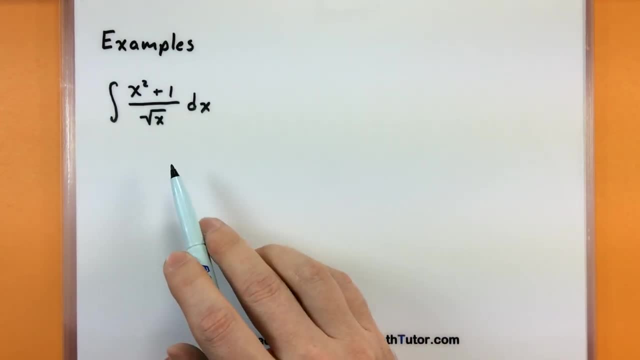 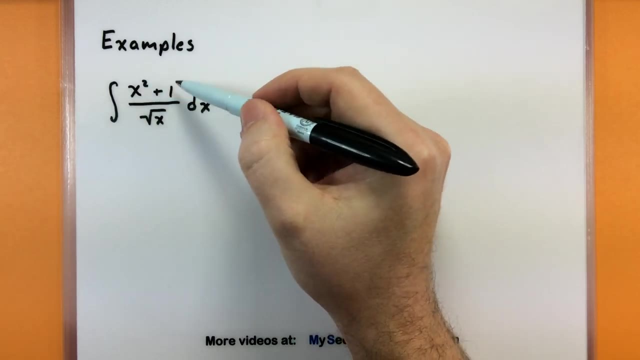 that can make this go a little bit better. Now, with this one, you have to be really careful how you apply your antiderivatives, how you work backwards, because you know I have something divided by something else. but if you think all the way back to those rules for indefinite integrals, 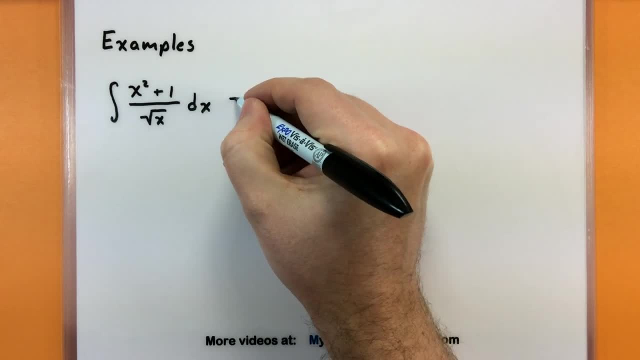 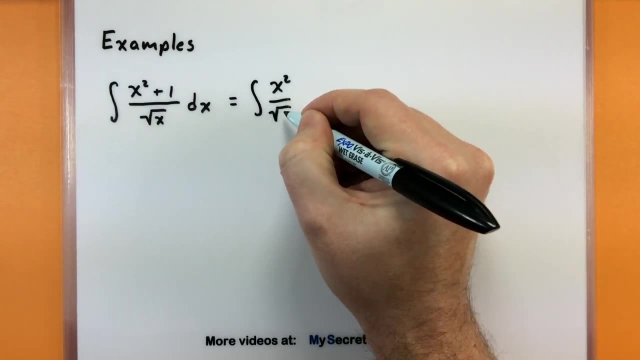 they said nothing about division. So for problems like this sometimes it's best to actually start rewriting them, And in some of my derivative videos this was also a handy technique. You know, if you just change what it looks like, sometimes you can handle it fairly quickly. 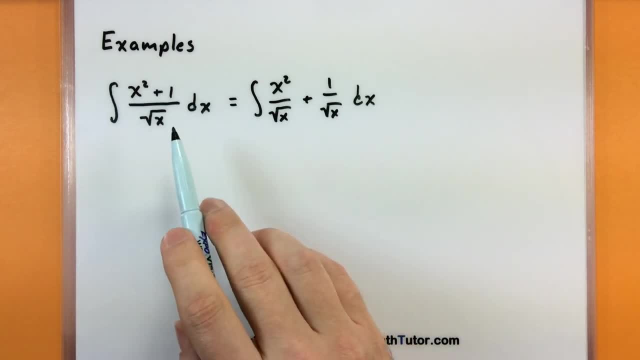 and use the rules that you actually have. So so far I've just split this up into two fractions. It looks a little strange, but it is a valid rule. You know, if we were to put these together, I'd make sure they have the same denominator. 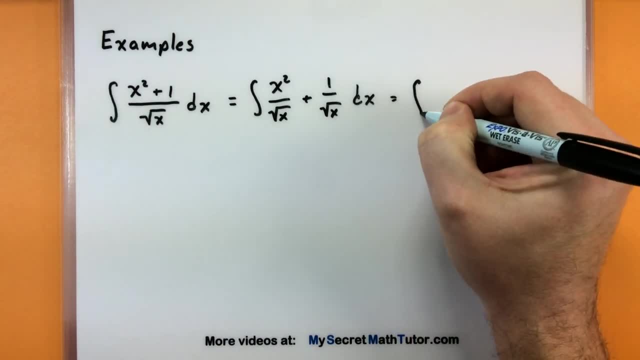 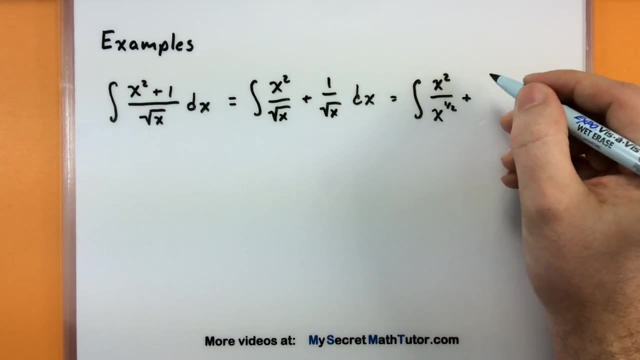 and sure enough, we'd end up back over here. Now let's see. moving on, I might look at this: instead of a square root, I would say this is like x to the one half. What I'm going to end up doing here is I want to reduce these powers. 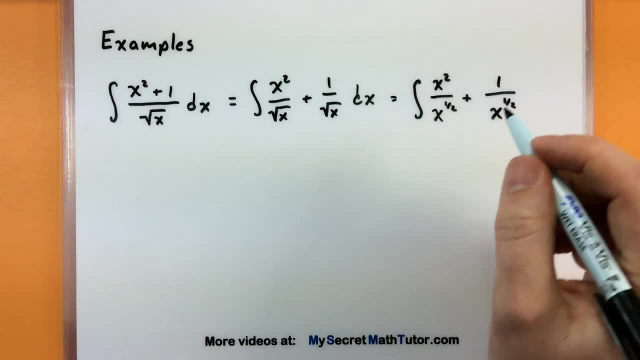 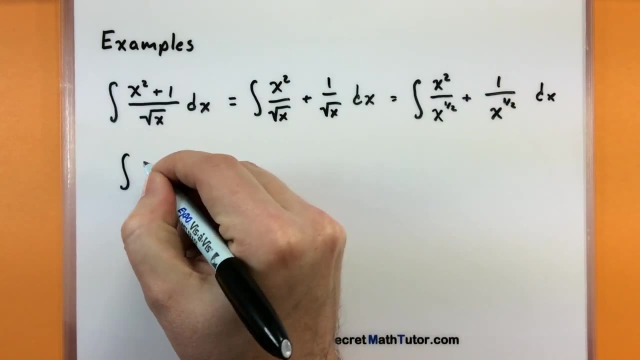 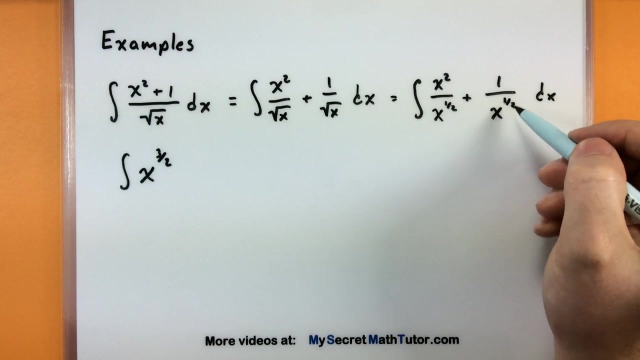 and so let's see, if I want to reduce this first power, I'd subtract the one half from the two. Let's see two minus one half. I'd be left with three halves. And here, since there's no x's in the top, 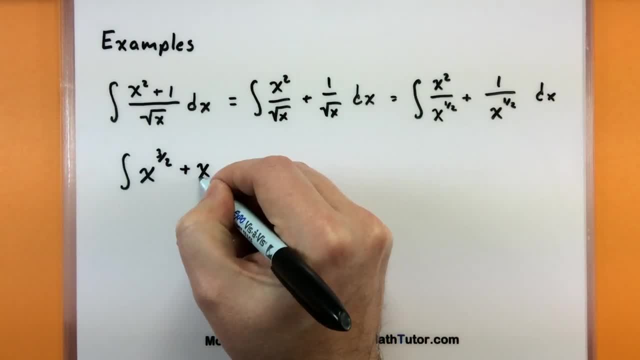 I can just consider this a negative exponent. so plus x to the negative one, half. So notice, we have not taken the antiderivative. I haven't even thought about that process yet. I've really just gone through a process of manipulating this so that I can start using some more of my rules. 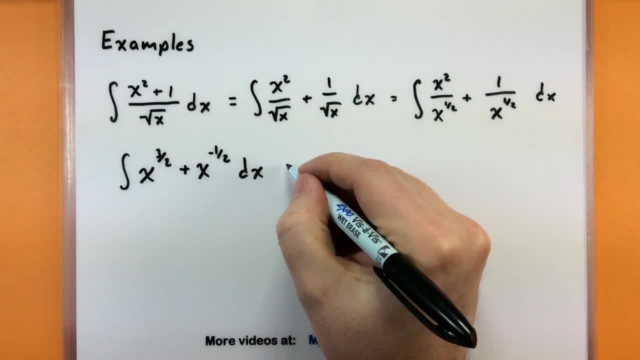 and now we can actually use that rule of adding one to the power and then dividing by the new power. So let's go ahead and do that. So I'm going to take my x, we're going to take the power that it is now. 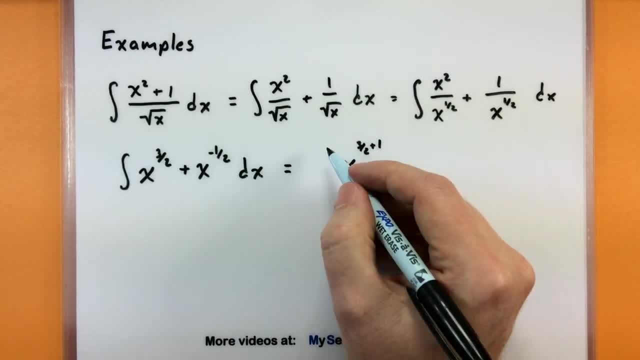 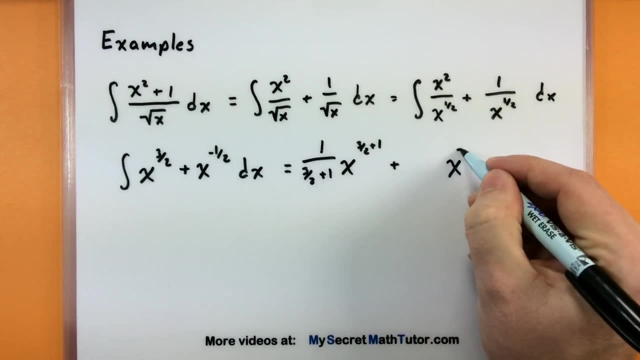 we're going to add one to that new power and whatever new number this is, we're going to divide by it. So of course, we have some work to do. That's what's going to end up over there, And we've got to do the same thing for this one. 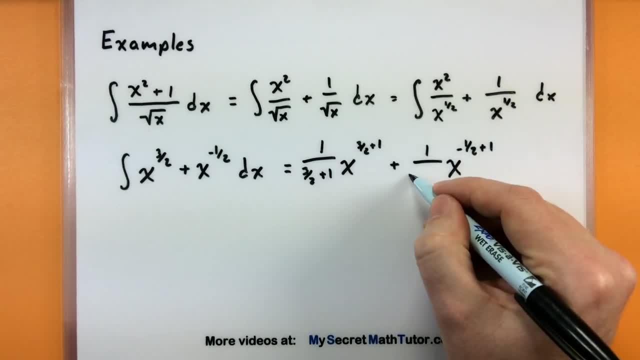 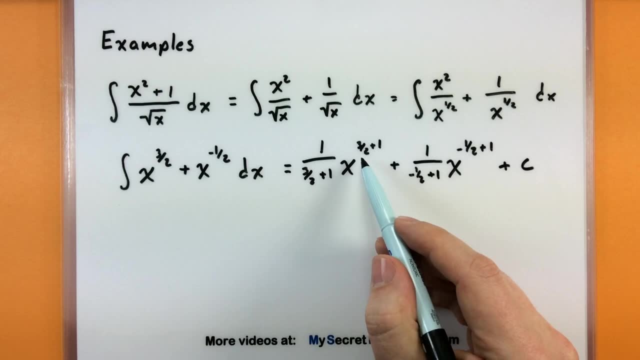 So negative one half plus one, and we're going to divide this by whatever new number that we get. All right, so that looks pretty good. We should probably put a plus c in there and let's go ahead and clean this up. 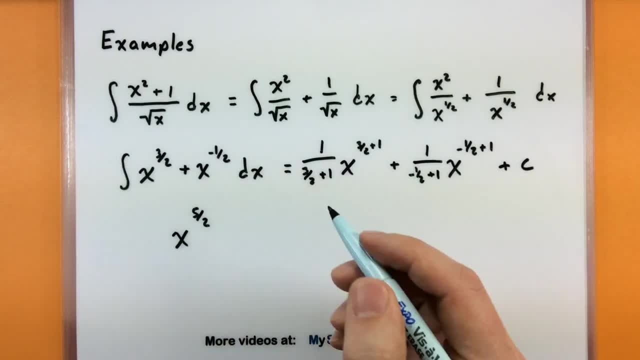 So three halves plus one, that would equal x to the five halves. So that's going to be this number down here, one divided by five halves, And let's see x to the one half. so negative one half plus one, one half, and that's this number down here. 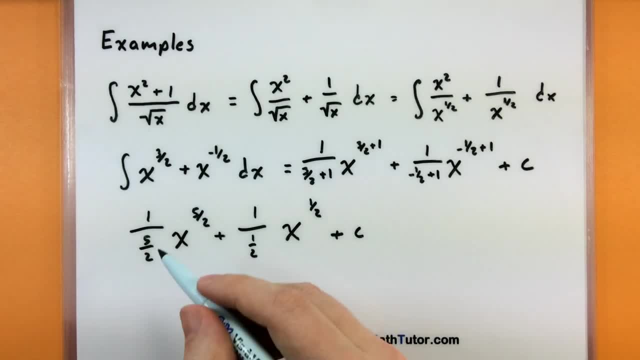 It looks a little messy and of course, we should probably clean this up. When we divide by a fraction, we want to flip and multiply, so let's go ahead and think what this is really doing. So this is one divided by five halves. 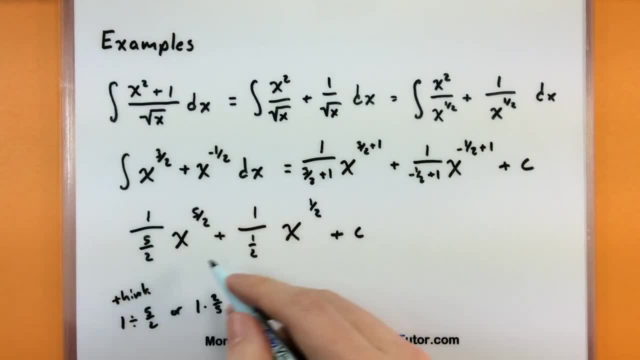 or we can think of it as one multiplied by two fifths. So this expression becomes two fifths multiplied by x to the five halves plus. we'll do the same thing here. this will be a two x to the one half. 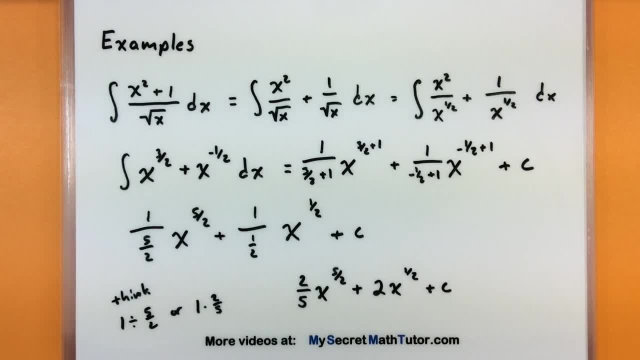 and we have our plus constant. Okay, so I had to really manipulate this thing so that I was only using the antiderivative of things that were added together and, in this case, just using a power rule to add one to the power and reduce it. 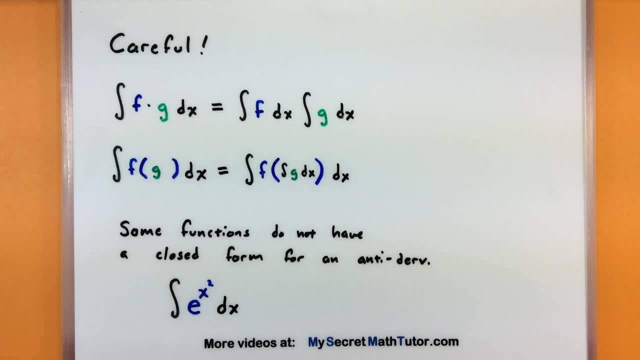 Now be very, very careful when you're doing antiderivatives. These are the most common mistakes that people will do. Sometimes you have two functions that are multiplied together and people will try and take the indefinite integral of each of those. This is not a valid rule. 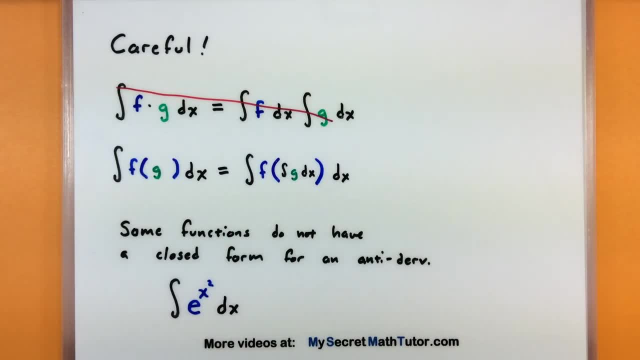 In fact you're going to handle that later on using something, a different rule for these antiderivatives. You'll get into u-substitution and stuff like that. Another one is what looks like a chain rule if you have a function inside of another one. 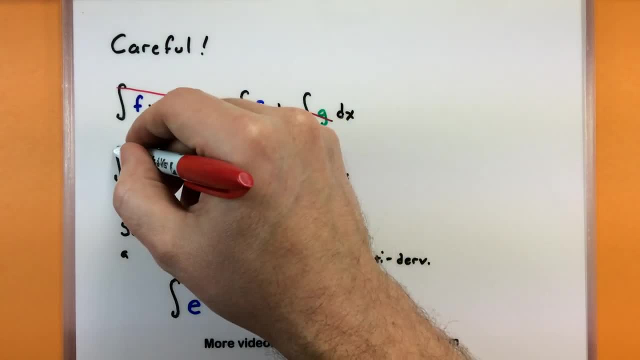 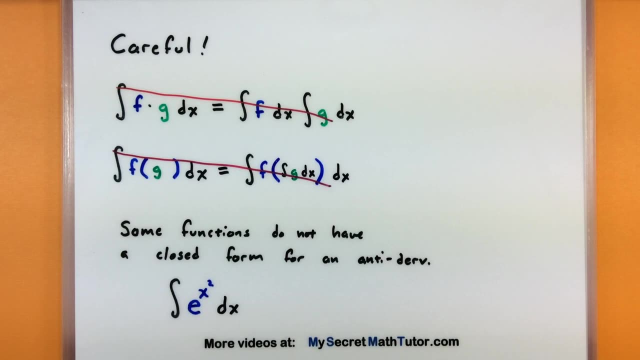 People will try and take the antiderivative of the outside and the antiderivative of the inside, but again, that is not a valid rule. You'll usually take care of those using something like u-substitution And, of course, the biggest rule, that. 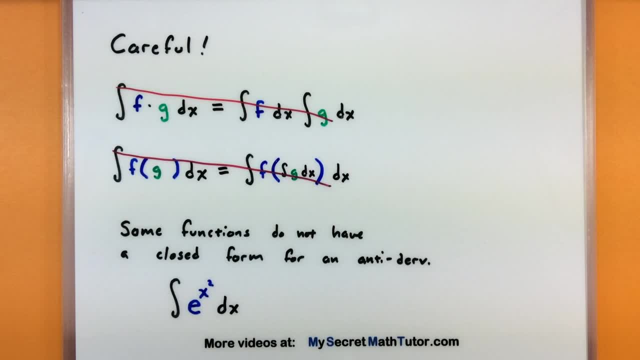 or not necessarily a rule, but the biggest problem that some people have with antiderivatives is even a very simple function might not have a closed form for the antiderivative. That means when I try and write down the formula or just write down what the antiderivative is. 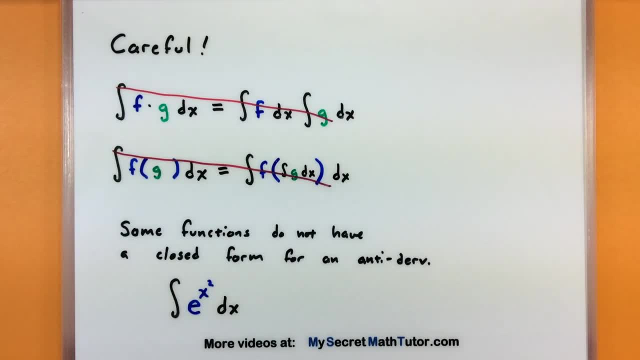 it's not going to be as simple as you think it is. It's not going to be a single finite formula that actually describes what's going on. So this one happens to be one of those that does not have a closed form, Even though it looks really simple. 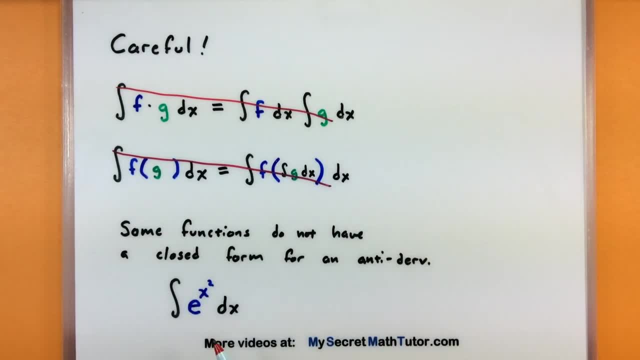 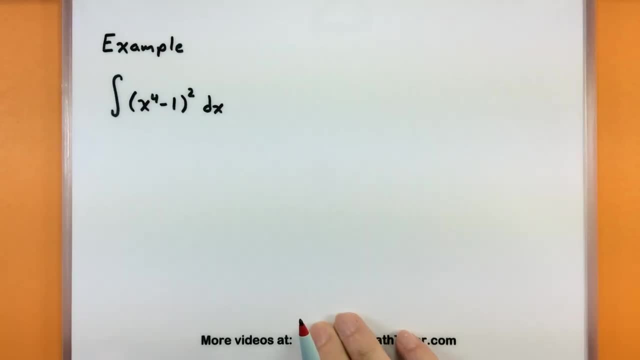 you'll probably have to wait until a little bit later in calculus to see what this guy's antiderivative is, and it's going to involve an infinite amount of functions, So be careful for those. Alright, let's get back to some ones that we can do. 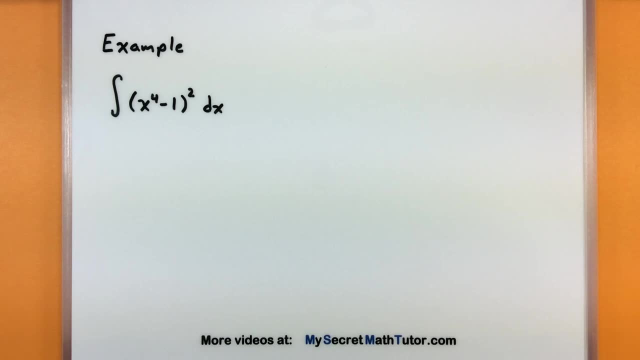 or at least ones that you know. it looks like maybe we can't do them, but again, if we manipulate them, just right, we have all the tools that we can actually take an antiderivative. Alright, let's try this guy out. 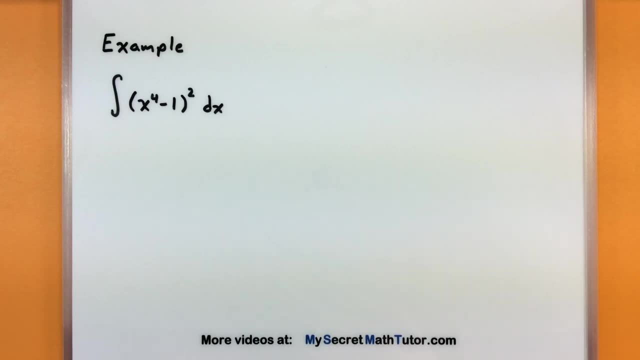 So here I have x to the fourth minus one, and all of that's being squared, And some common mistakes might be to try and add one to this power, divide by three and continue on from there. But we really have another function inside of that, okay. 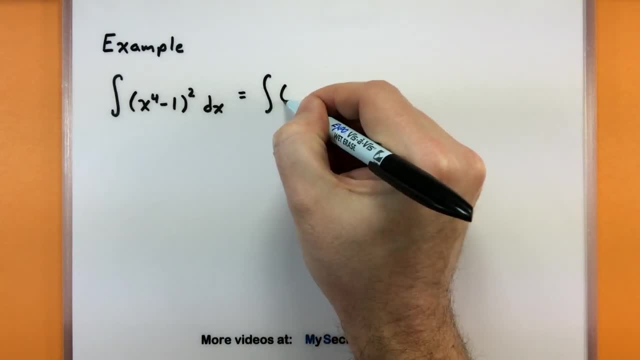 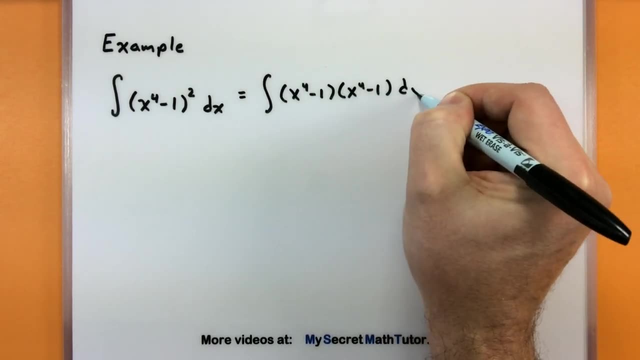 So we have to be a little bit more careful. We want to think of manipulating this first. I'm just going to spread this out: x to the fourth minus one multiplied by x to the fourth minus one- And I'm doing this so that I can expand it out. 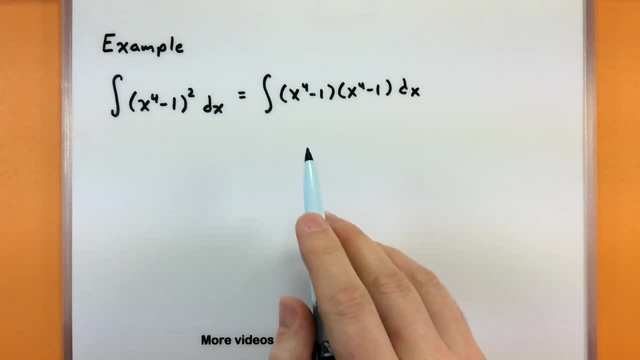 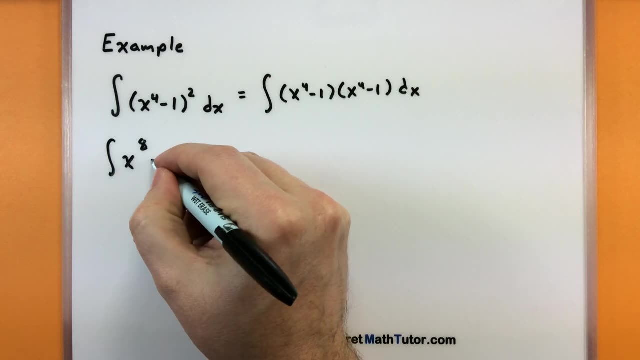 into a whole bunch of functions that are added. then we'll go ahead and take care of those, Alright, so let's keep expanding x to the fourth times, x to the fourth. we'll add those exponents. Outside will be minus x to the fourth. 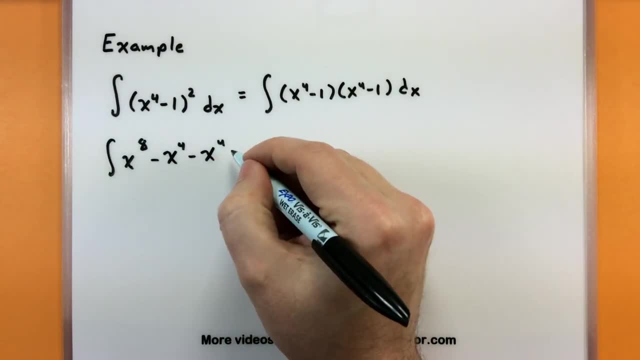 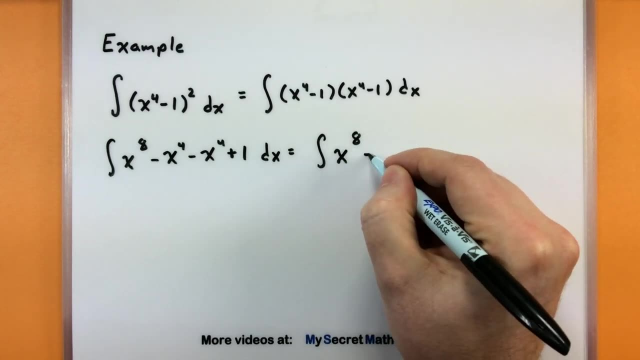 inside: minus x to the fourth. Last terms, minus one times, minus one plus one, And let's go ahead and combine the common terms from here. So x to the eighth minus two, x to the fourth plus one. Okay, that's all good. 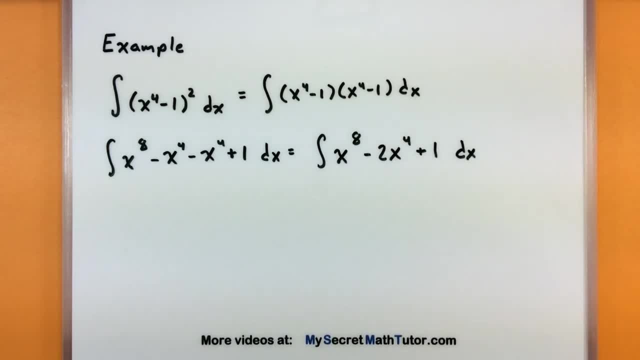 Now that it's all spread out, now I can worry about actually taking this antiderivative And of course we'll just use a power rule. So, starting with the first one, eight plus one is nine. We'll divide by that new power.